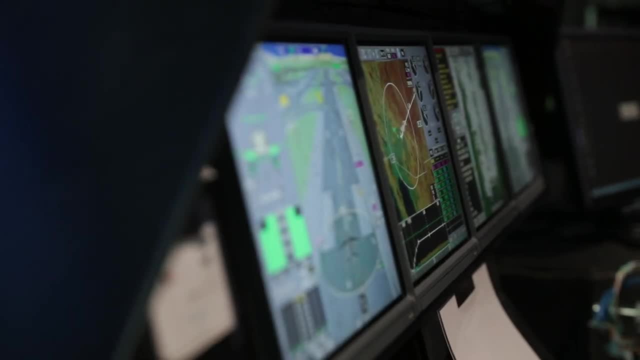 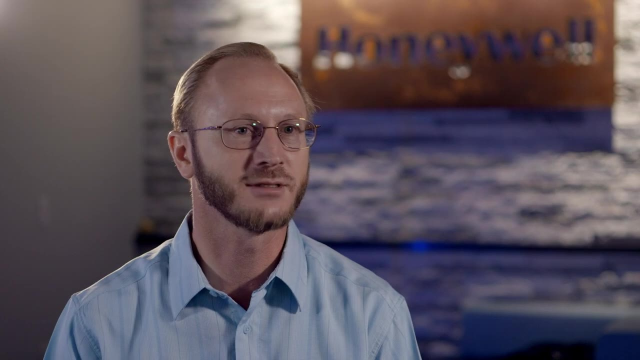 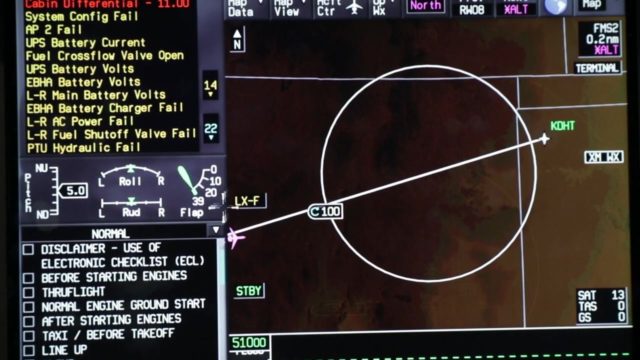 dealing with the intricate details of each individual component, but it's more looking at the big picture. Some people would say that we would deal with the forest instead of the trees. It all works together to give us the complete systems view of what we do here at Honeywell. Being a certified pilot enables me to understand. 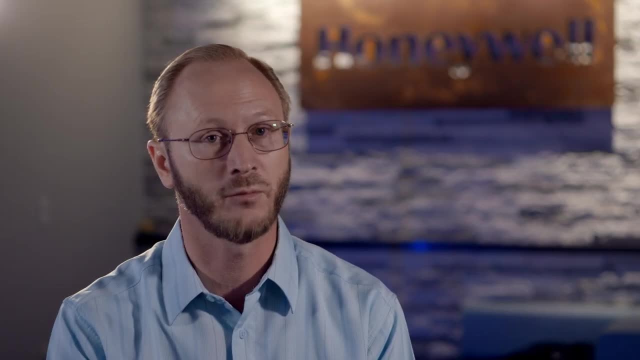 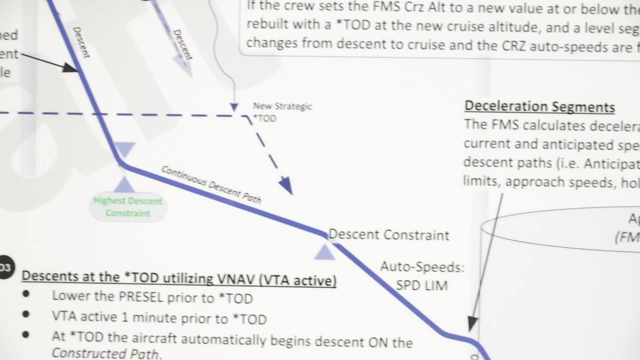 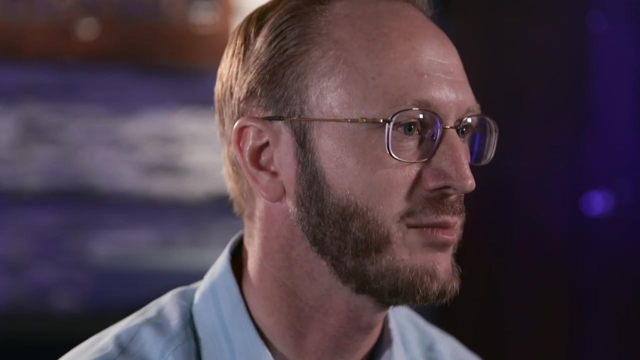 what the pilot's actually asking for. In many cases we hear some of that pilot's request from an engineering perspective. What is the intent of their question? Interpret that into a function that we can offer up to them, and that product becomes more than what they anticipated Once. 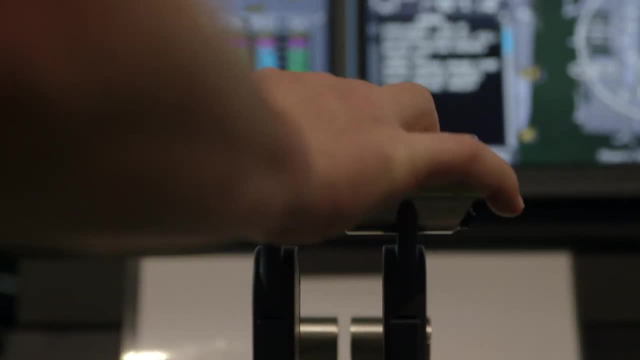 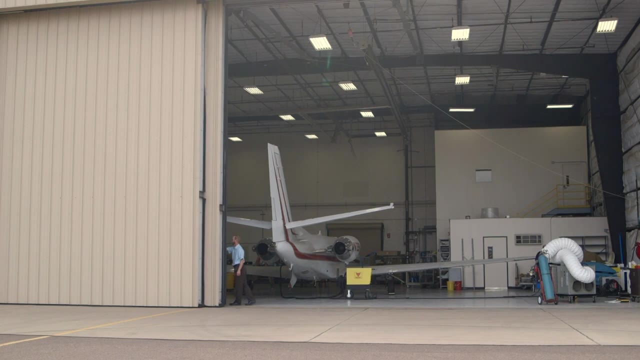 it has proven itself. it's time to take the next step. I'm Steve Smith and I'm a systems engineer. If we're going to put this pilot on our system, only then will we actually put it on an aircraft and take it up for test flight. Our job is never finished. We need to always be ready for change. 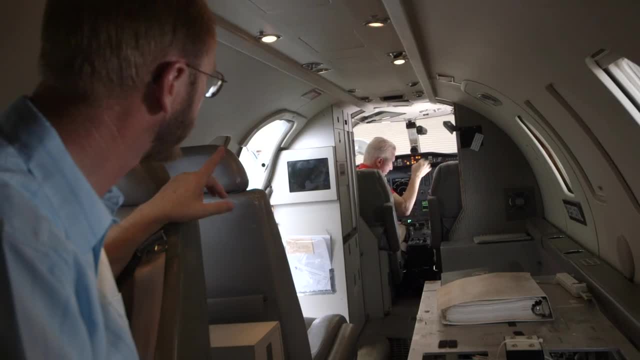 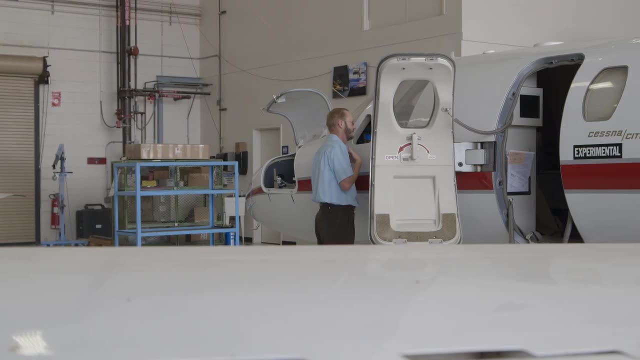 ready for a better product. If you look at the maintenance page on that system up there, We're all about presentation and improved workflow. to make the pilot's job easier and the whole flight safer, We could host an EFB type app. Being a perfectionist at heart, I want to see this. 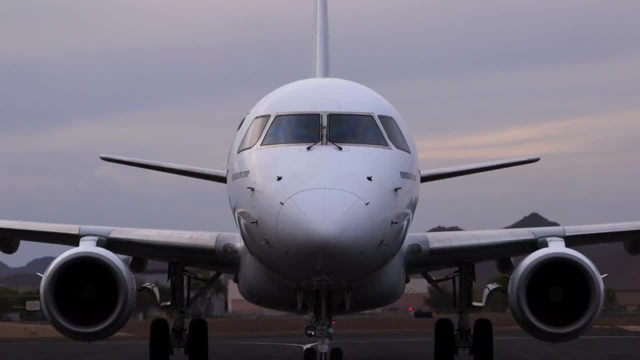 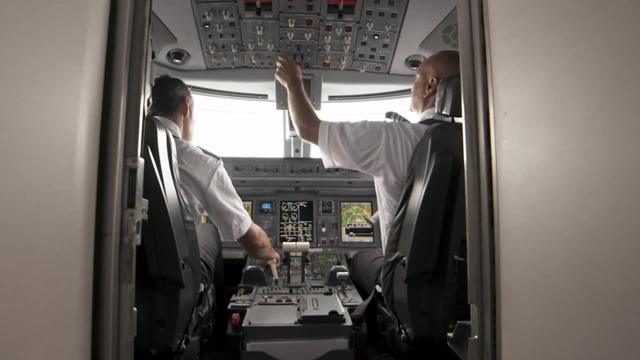 product better to continually improve on it. Seeing that happen over the past almost 20 years now is a driving force for me. To see the product in use, to see the pilots using it, actually using what you have created, that's a very rewarding feeling. 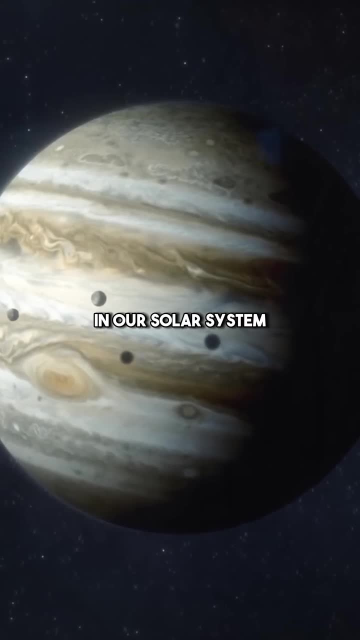 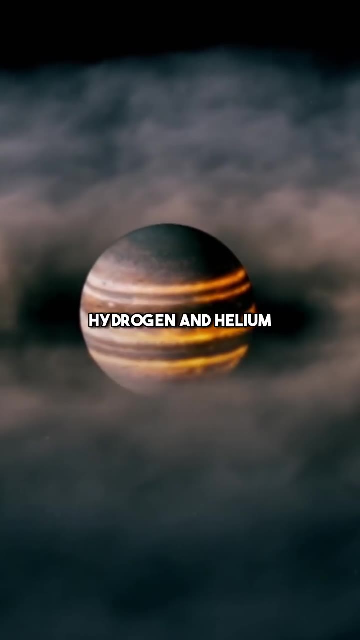 Have you ever wondered why Jupiter is so much larger than the other planets in our solar system? It turns out that Jupiter is not a typical planet, but a failed star. Jupiter is composed primarily of hydrogen and helium, just like our sun. Astronomers believe that when our solar system 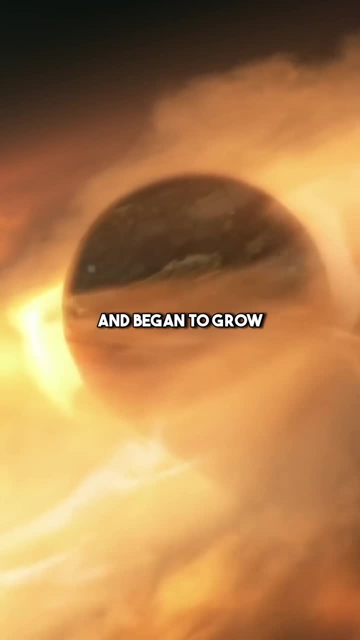 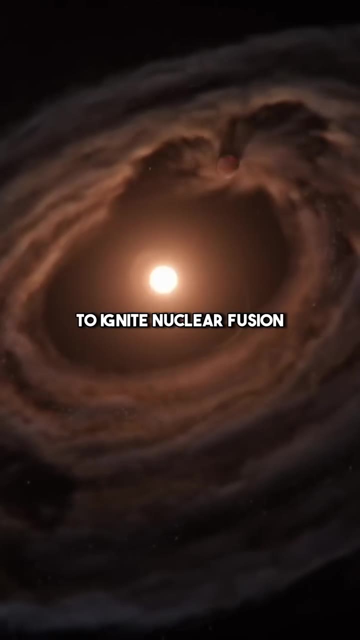 was forming, Jupiter started to collect dust and gas and began to grow, But it never got big enough to become a star. If Jupiter was about 80 times more massive, it would have been hot enough and dense enough to ignite nuclear fusion and become a star, But instead Jupiter ended up as a gas.